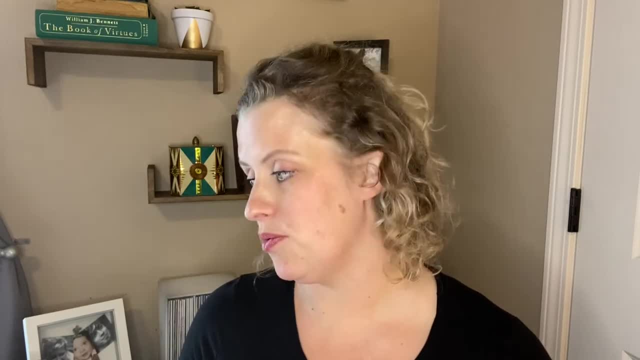 you do not need any workbooks, So there is very minimal writing involved at all. Most of the workbooks are not very thick, So you don't need to have a lot of workbooks. Most of the workbooks are not very thick, So you don't need to have a lot of workbooks, So you don't. 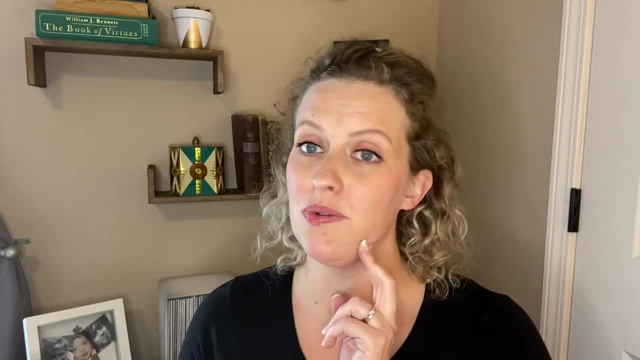 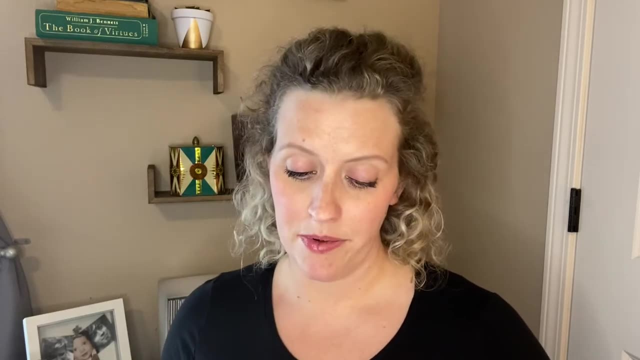 need to have a lot of workbooks, So there is very minimal writing involved at all. Most of the writing exercises are optional and I choose not to do them usually because we do a lot of writing with the Writing with Ease program, So this program is completely scripted, like most of 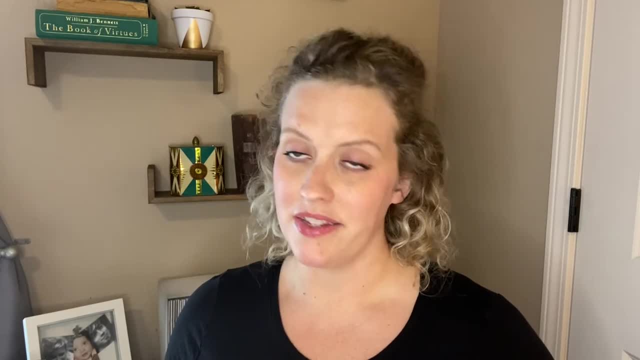 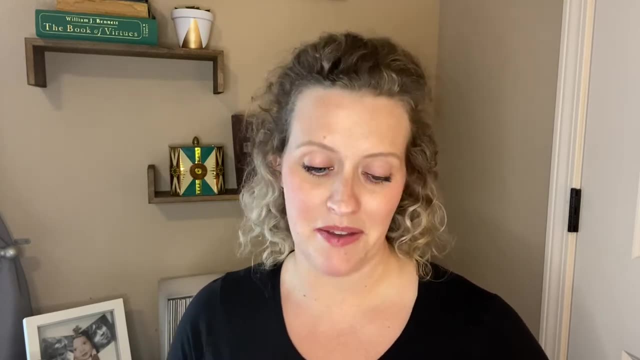 well-trained mind things are, And that is super easy for me. I don't have to worry about how I'm going to teach something. It tells me exactly what to say and what my kids are expected to say back to me. So this goes over your typical grammar. So we're talking punctuation. 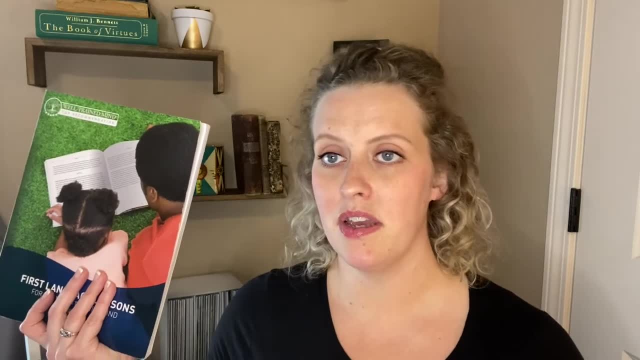 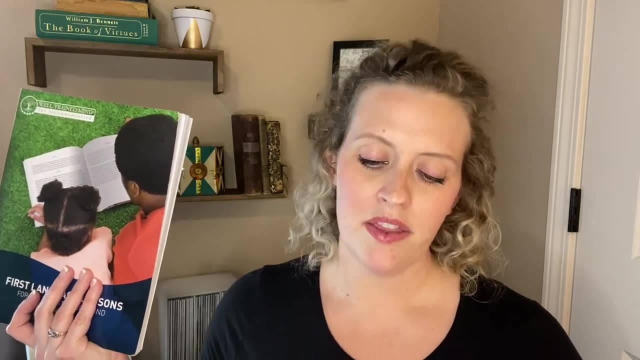 parts of speech. proper nouns, common nouns, abbreviations, when to capitalize all of that basic stuff that you would think of when you think of basic grammar. Then there's also, like I said, some copy work. We don't do much of that because 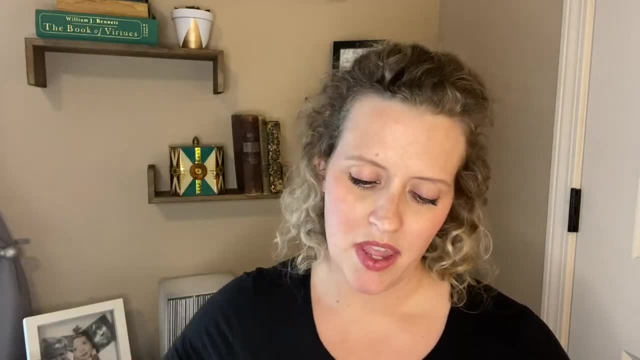 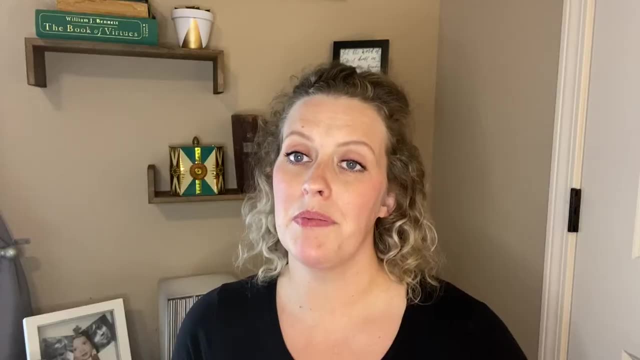 we have copy work with our writing program. And then there's also some narration. Sometimes you look at a picture and are asked questions about it. Sometimes you read a story or a poem and answer questions about it. Then there is also some poetry memorization, which is very helpful. 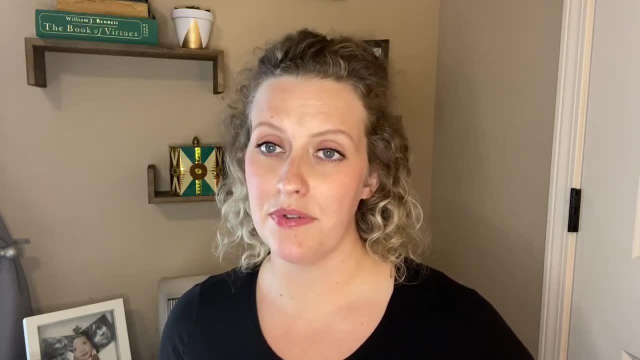 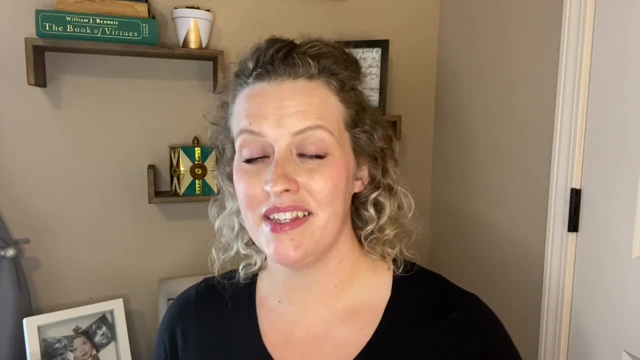 And all of it is based on really good literature. When they, when they use examples, they take them from really well-written literature, which I always love. Now my son is in second grade and just on level one, which they say is a totally acceptable way to start this program. 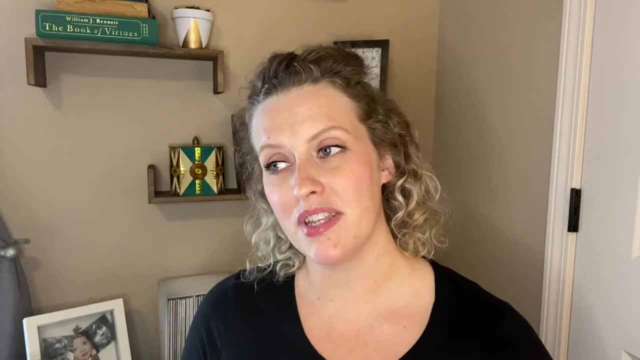 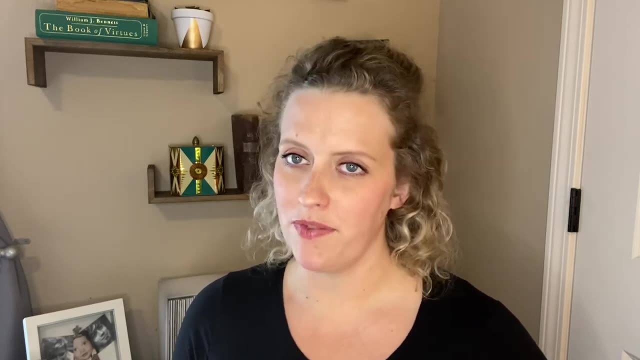 You don't have to start level one in first grade. We did that with my older son and I kind of regretted it. I really regretted it with the writing program. I didn't regret it as much with grammar, but I think he definitely could have waited another year. 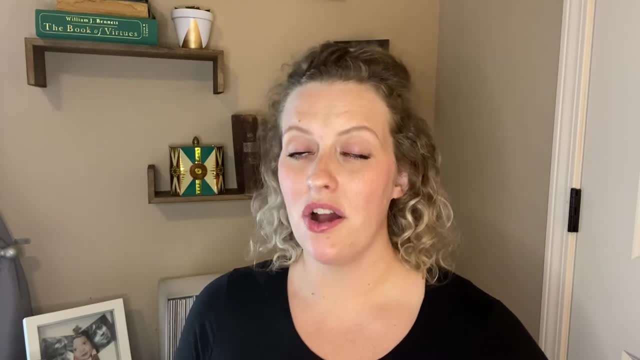 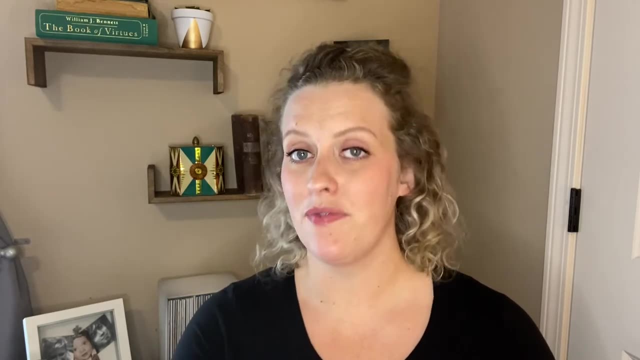 So with my second son, I didn't want to make the same mistake, especially because he's an August birthday, So I went ahead and started him on level one in second grade, And he will be using level two next year. So let's flip this camera around and I will let you see inside it. 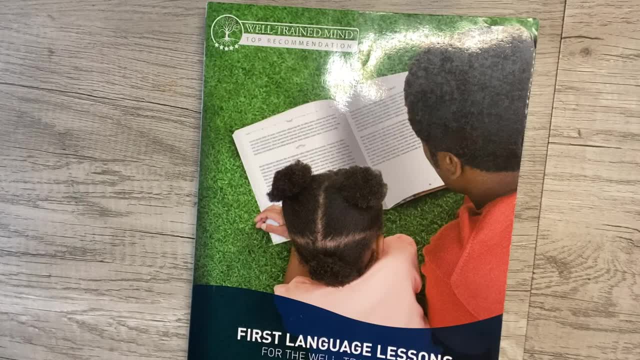 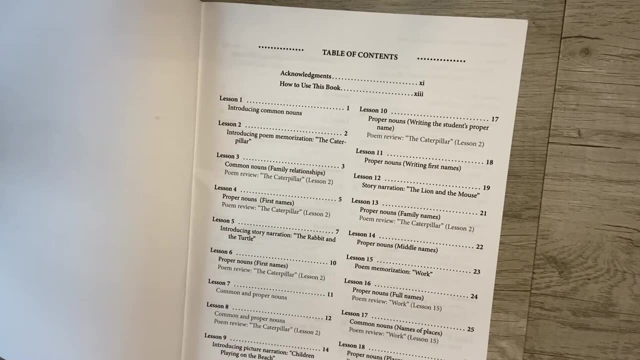 All right, level one. here is your cover. I know this is pretty zoomed in, but I want you to actually be able to take a look and actually be able to see what is in there. Here we have our table of contents that tells you exactly what you will be teaching in each lesson. 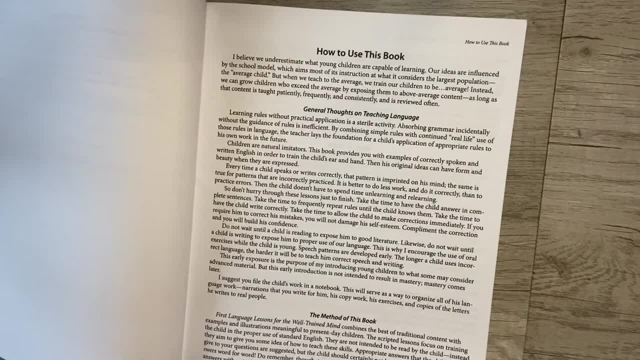 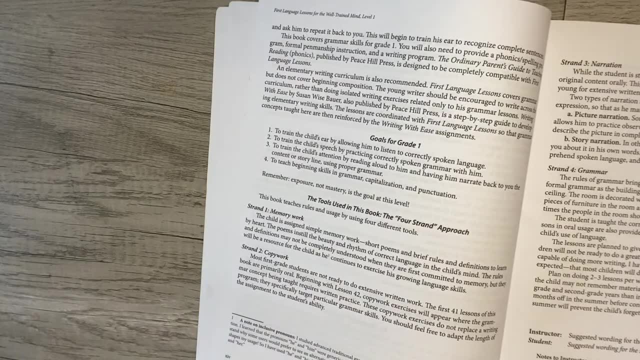 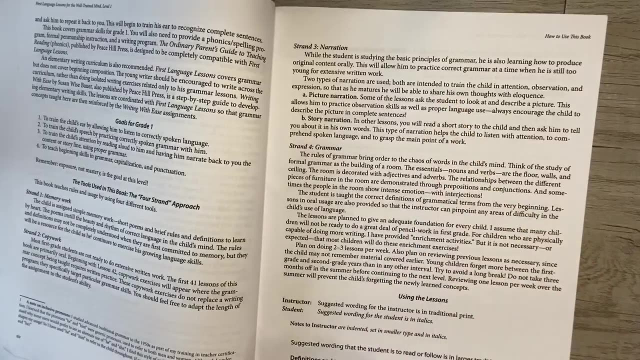 Here are the acknowledgments And here is an overview of how to use the book: her general thoughts on teaching language, the method of this book- Here you'll see the goals for grade one. And then she talks about her four strand approach, which is using memory work, copy work, narration and grammar. 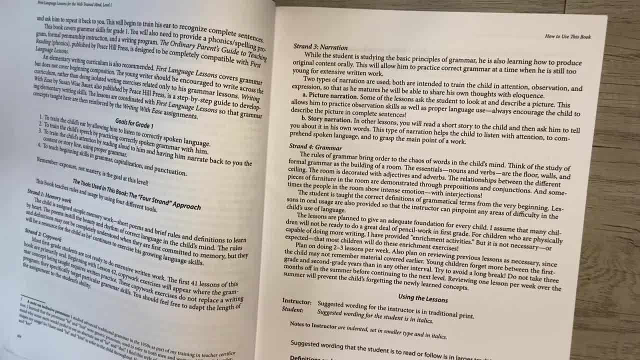 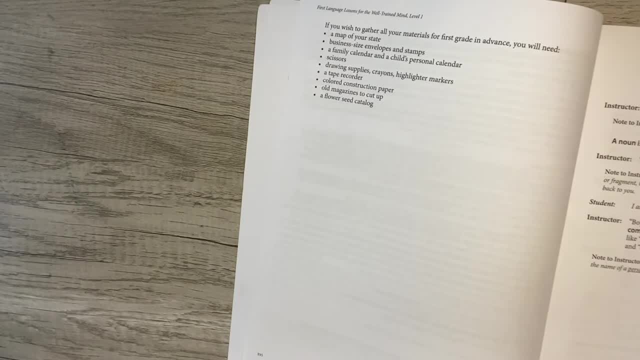 And then it gives you a detailed breakdown of how to use the lesson, And then here you will find a list of things that you will need to teach throughout the year, And let me just tell you there's a lot of these I never used, so you can do it without. 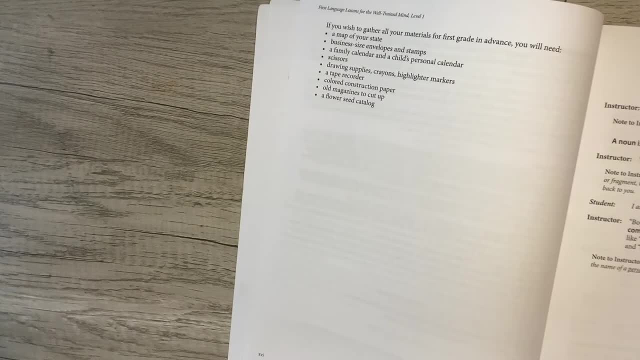 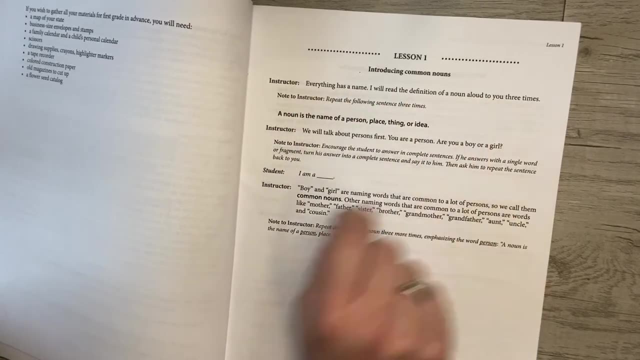 However, I'm sure they are useful if you do decide to use them. Here's a look at lesson one. So here is what you say. Here is what you say together, Again what you say, what your students should say, what you say. 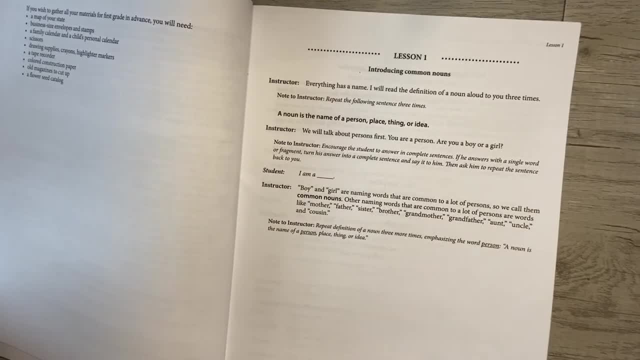 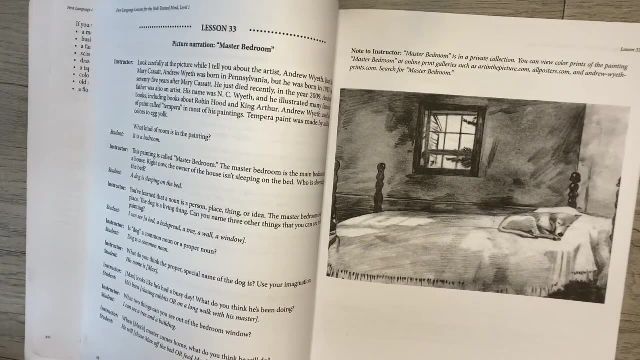 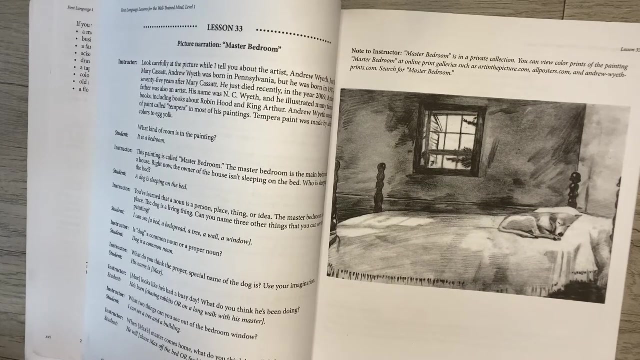 That's the lesson. Typically, I do three lessons a week in order to get through this all in one school year. Here's lesson 33.. I wanted to show you kind of what a narration page would look like. So here is the picture that you have your student look at and then you kind of tell them about it. 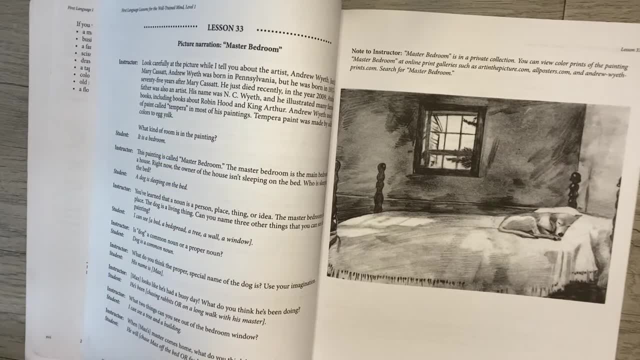 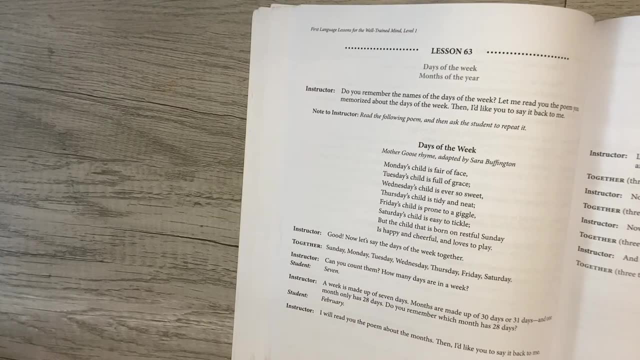 Again all scripted, And then you just do a back and forth dialog on having them really explore the picture and tell you in their own words about it. Here in lesson 63 is an example of a poem that you will need to memorize or have your student memorize, rather. 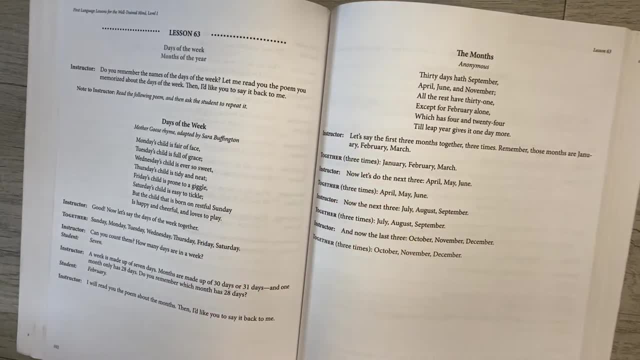 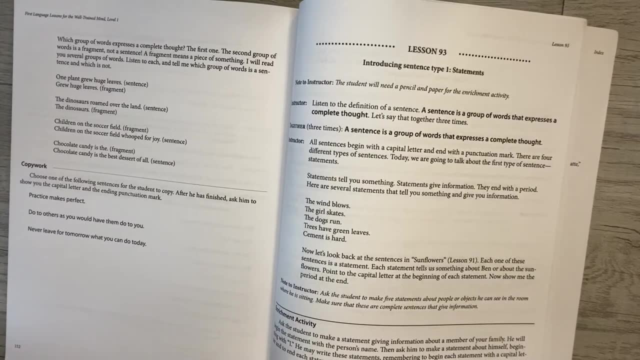 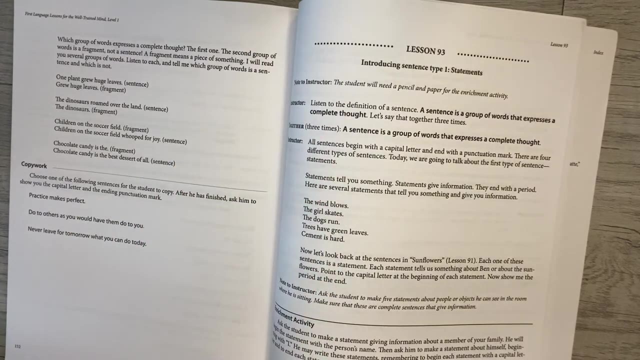 And here's another one, And then the different dialog you will need to have following that. And all of these lessons are fairly short. Some are shorter than others, But none of them are super, super long in this level. So here you're going to be introducing statement sentences. 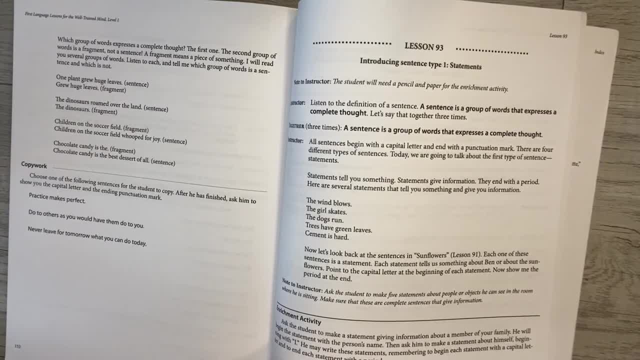 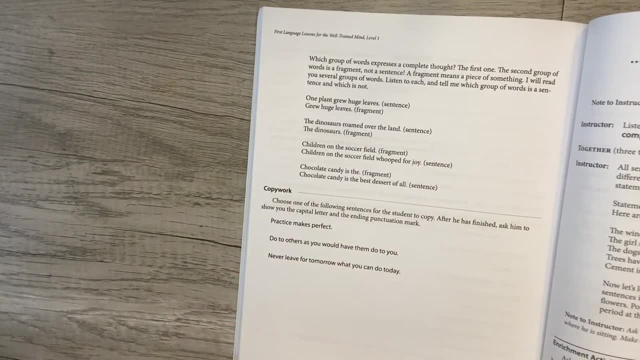 And then every once in a while, you'll have an enrichment activity. We sometimes do those, sometimes don't, But, like here in the lesson before, there's an example of copy work and we just don't usually do those. And then here at the very end, is your final grammar review. 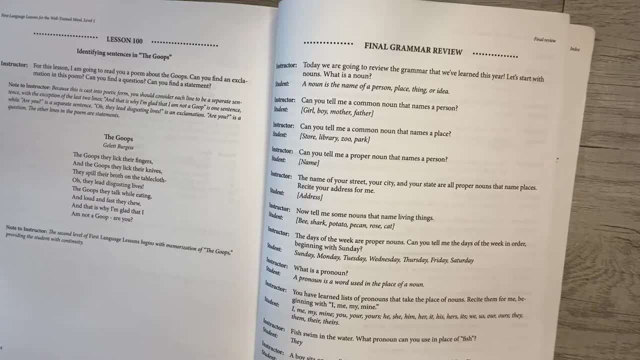 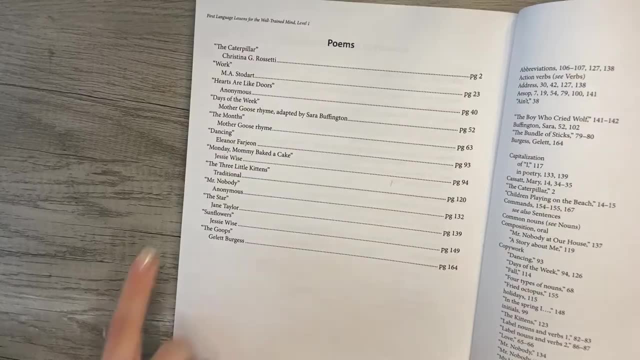 So it's just all discussion. It's not any sort of test or anything, But you just talk about basically everything you've learned over the course of the year, And then here is your glossary of terms and definitions. This here shows you where you can find all the poems that you're going to memorize throughout the year. 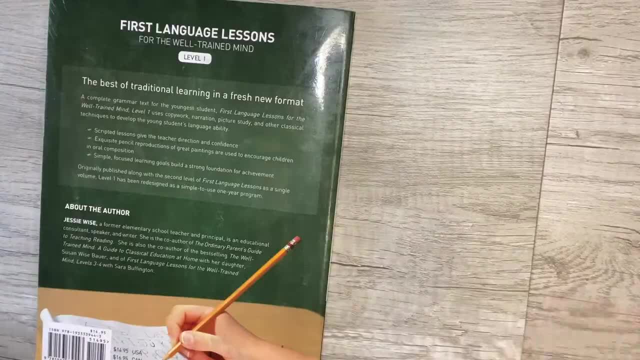 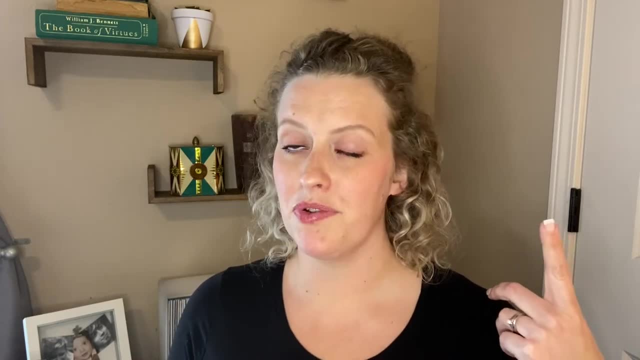 The pages that they're on. Here is your index. Okay, hopefully that was helpful. Now be sure to check out, if you haven't already, my Ordinary Parent's Guide to Teaching Reading. flip through and review, Because this is also by The Well-Trained Mind. 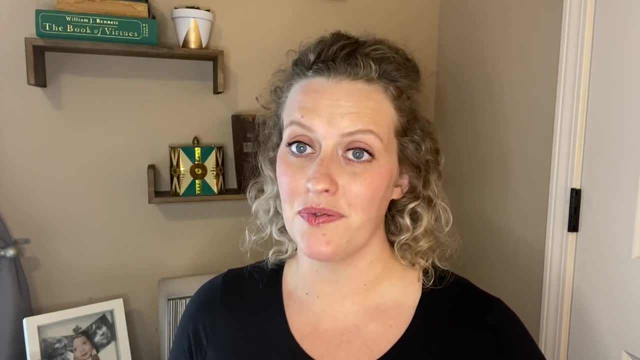 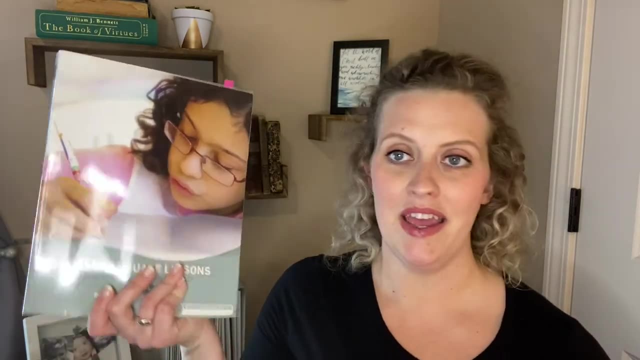 And it has helped both of my boys learn to read very, very easily. So, for level four, this is what we're going to do. This is what my fourth grader is using. As you can see, this is a lot thicker book. 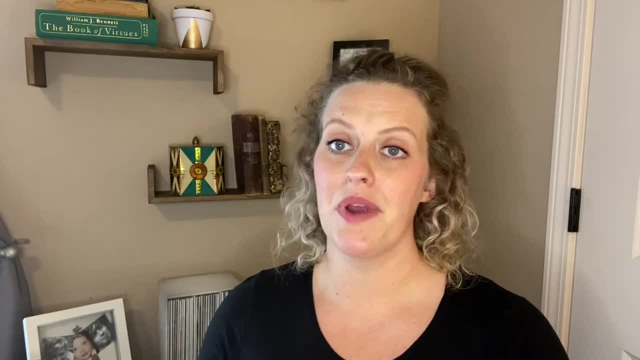 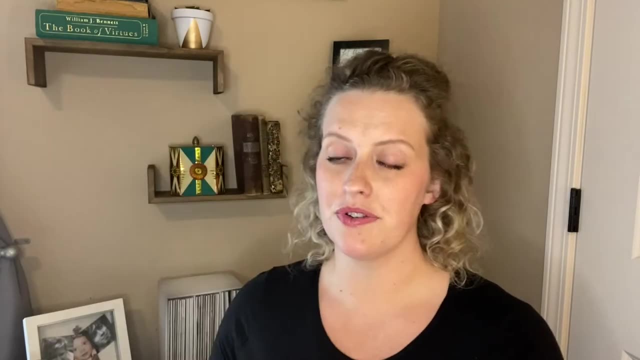 It's a pretty hefty book, But this walks through every single thing. This serves as both what you teach from your teaching text and your answer key, So the answers are built right into the lesson, so you don't have to have a separate key for that. 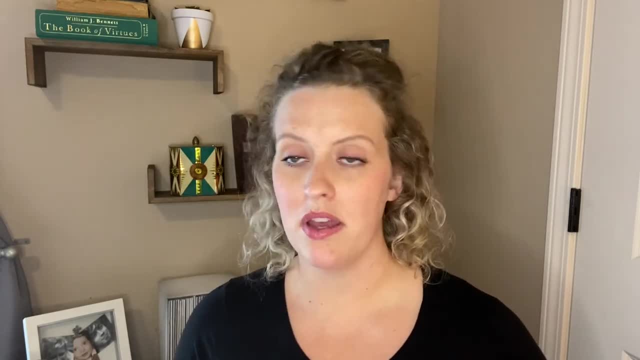 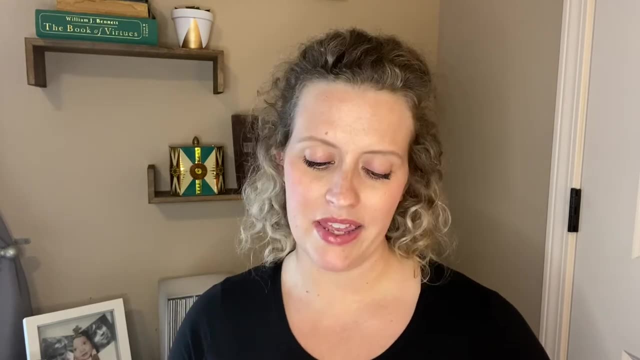 And levels three and four. you do need to have the student workbook. I don't have that to show you because in the beginning of the year I cut the bindings off and put them into my file box system. Again, this is totally scripted. 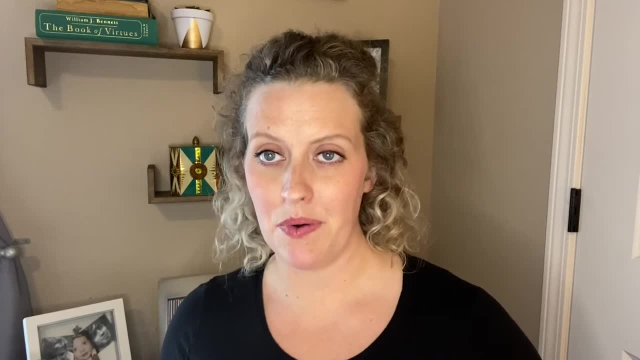 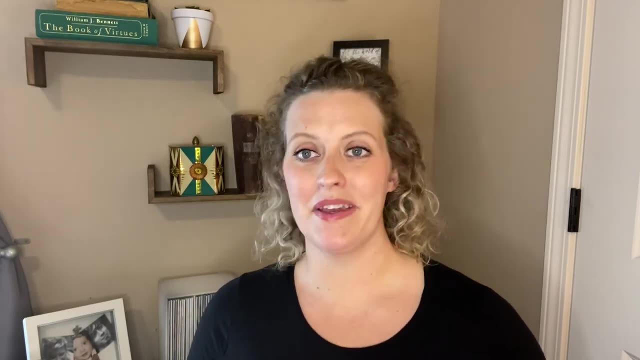 For us it is almost a little too thorough. Now, the only reason I say that is because sometimes the examples are excessive, And so sometimes I'm like, okay, if you do two correctly, then you don't have to do any more. 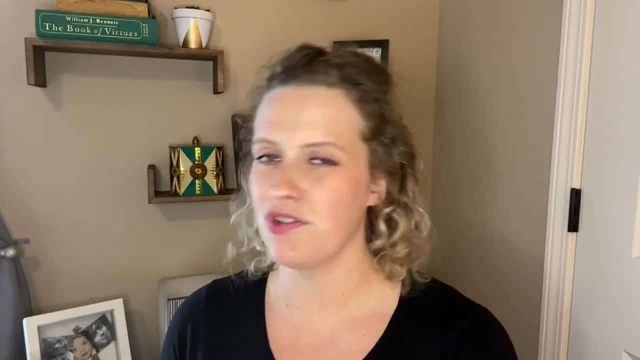 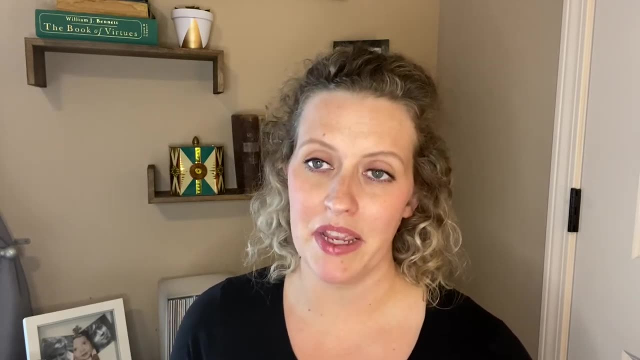 Or sometimes there's just like here's the correct way to do it, Look at it and then copy it And I'm like, okay, well, if you can just read these out loud to me and kind of point to the certain punctuation that we're talking about, 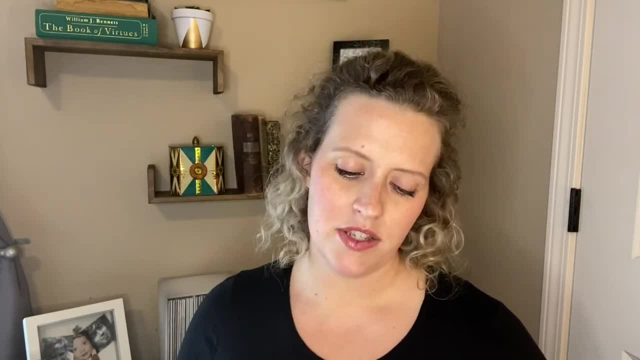 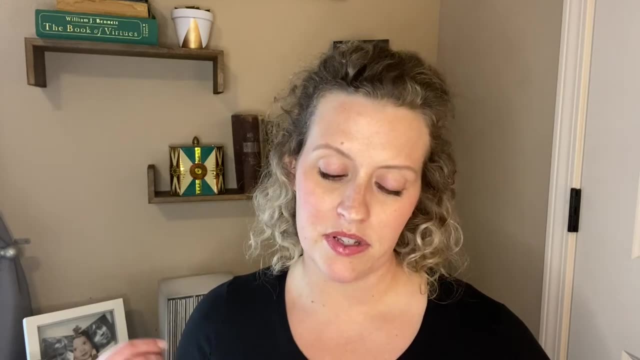 or capitalization or whatever it may be, Then we'll call it good. So in here it does review- you know your punctuation and your parts of speech- and actually goes into those a lot deeper. And then there's conjugating, there's poetry, there's proofreading. 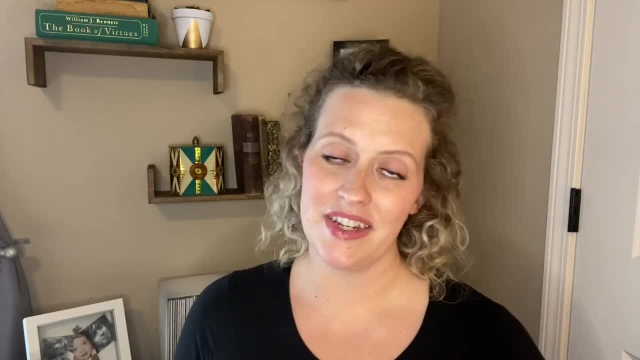 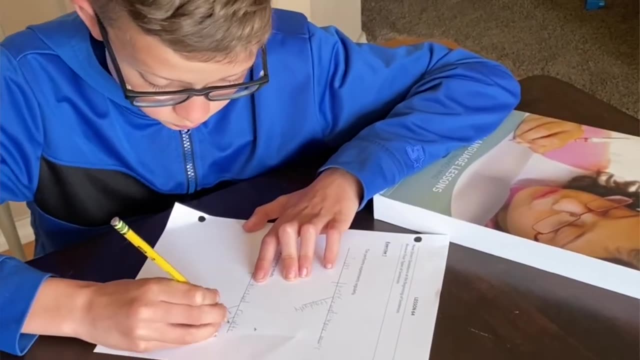 And then there's a lot, a lot, a lot of sentence diagramming, So we're really breaking down those parts of speech and seeing what parts of the sentences are what, And my son is actually really, really good at this, which I find interesting because he's not a great writer. 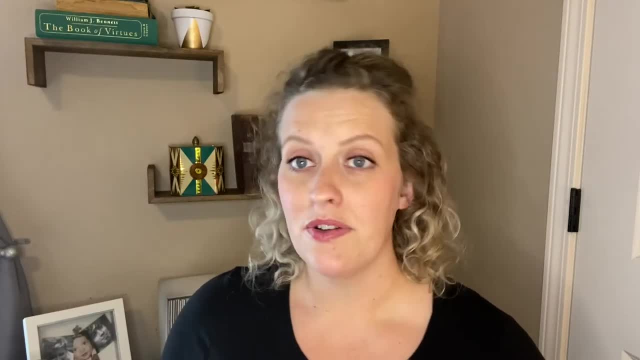 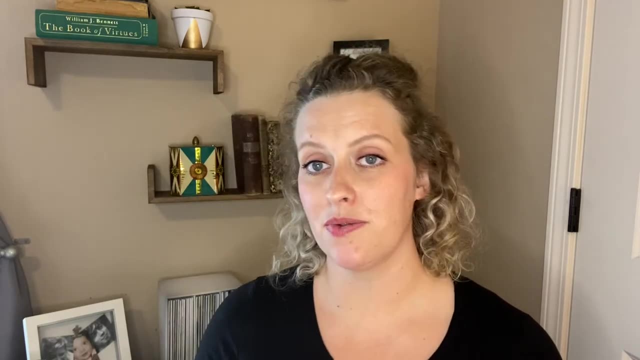 He doesn't love writing, but he's really good at grammar. And then there's also extra units at the back And they tell you you can either just save those all for the end and do them at the end, or they give you a schedule to use where you can just split them up evenly throughout the year. 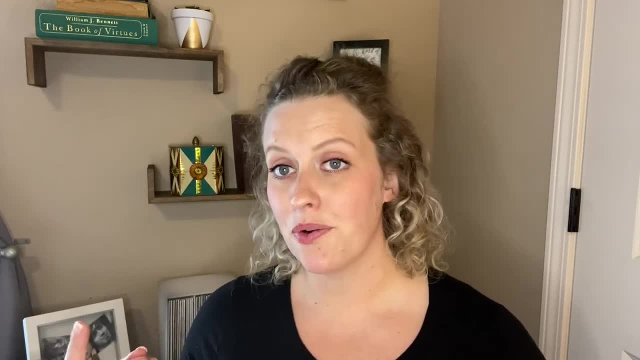 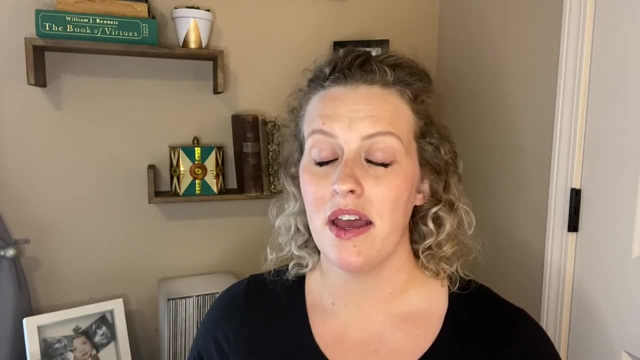 which is what we've chosen to do, And those are letter writing and dictionary skills. So where you learn how to read a dictionary entry, how to look up dictionary words in a dictionary, which I know is kind of a lost art, I feel like Google's there, right. 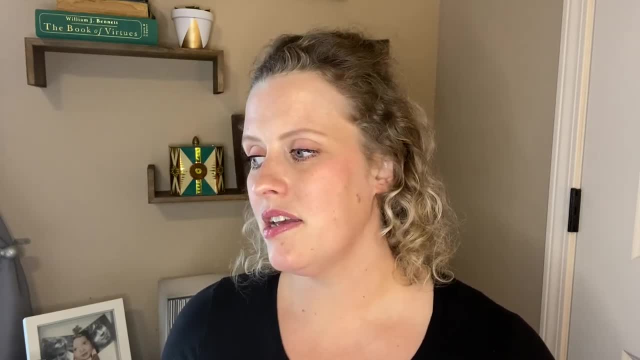 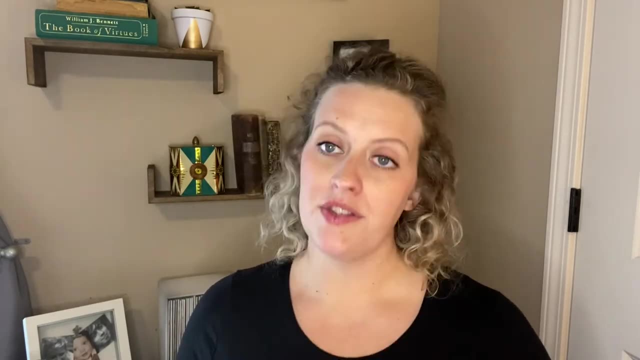 But I think it's an important skill to have And Being able to understand, when you do see a dictionary entry, what the heck all of those symbols and letters and weird things mean. So, as I said, we use this all four years with my son this next year and maybe in sixth grade. 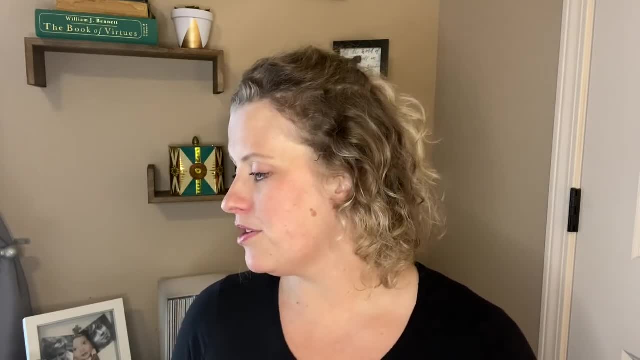 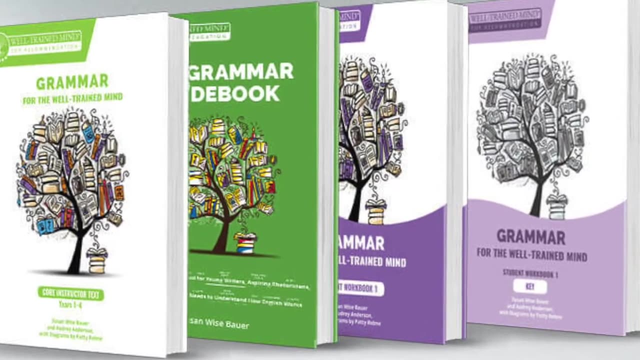 Also, we will be taking a break from this, because here you go into an entirely different program they have for middle school and high school And they say you can start it as young as fifth grade. but the fifth grade is pretty young And so if you do start it in fifth grade, you have to start really, really young. 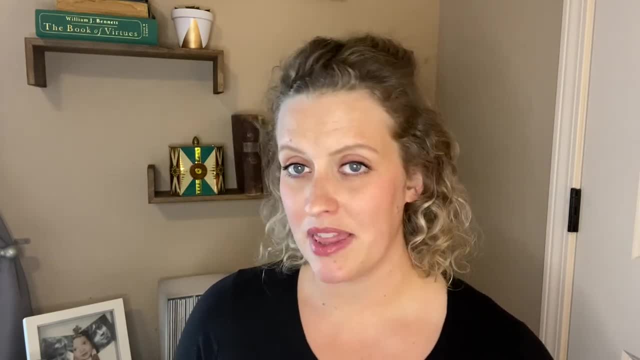 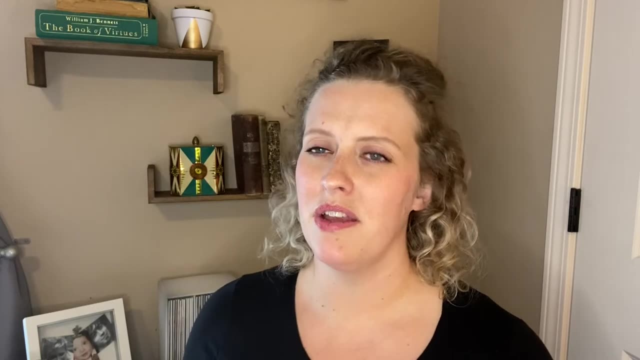 You have to start really, really slow. So instead of just doing that, I thought we would take a year or two and kind of just try something else for a while, Not because I don't like this program, but just because I don't want to stretch him too much next year. 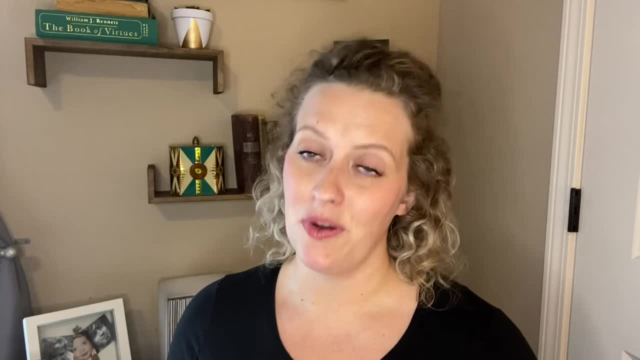 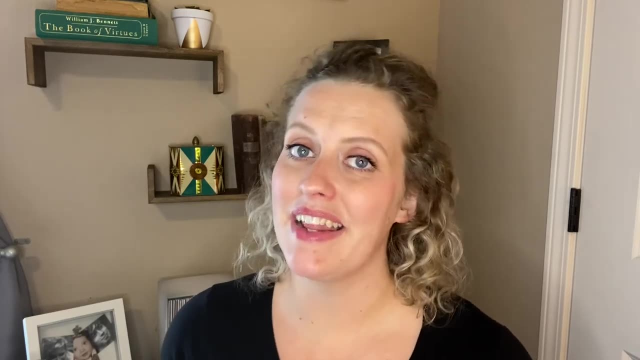 There's already a few things that are going to be changing next year for us, and I don't want it to be overwhelmed for him, But we will be coming back to this probably in seventh grade. So let me take you on a look inside level four. 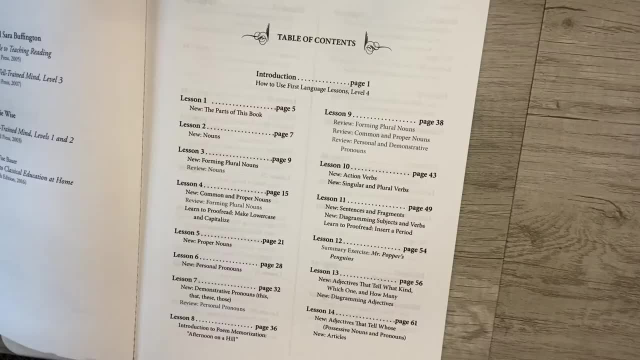 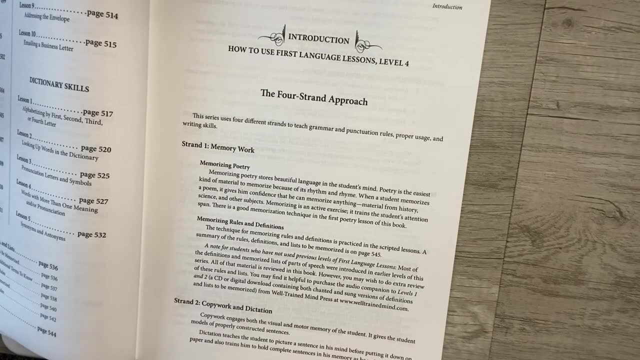 Here is our level four cover. Here we have your table of contents again, where it just shows you each lesson. It just shows you each lesson what you will be teaching. And here is your introduction, where again it talks about the four strand approach. 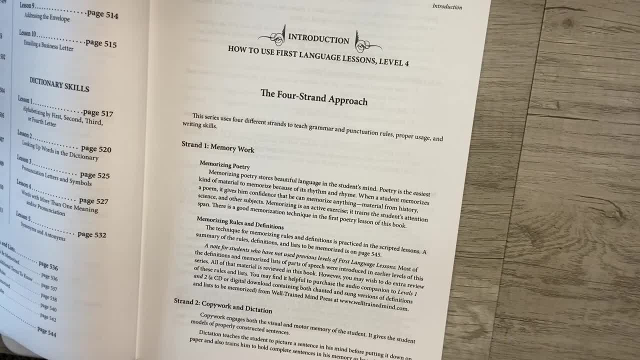 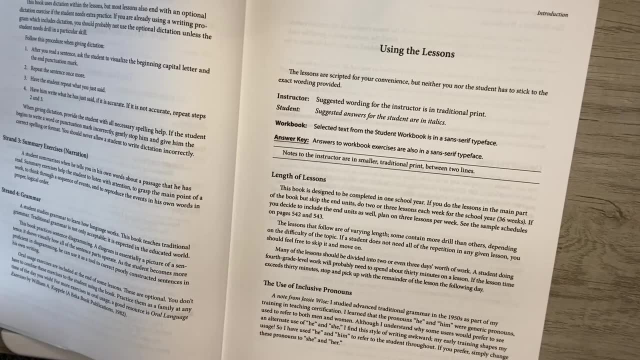 which it told you about in book one, and I'm sure it's in book two and three as well. And then here it tells you how to use the lessons. It tells you the length of the lessons. It says to do two or three lessons each week in order to complete it in 36 weeks. 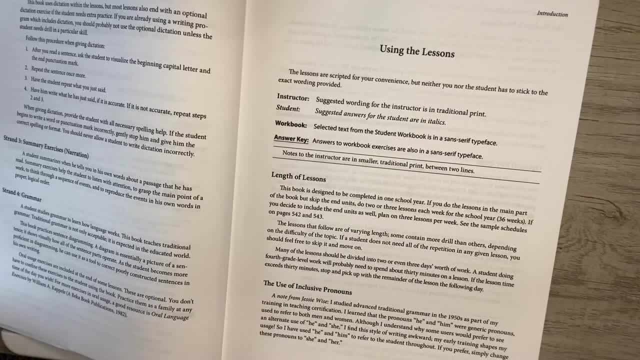 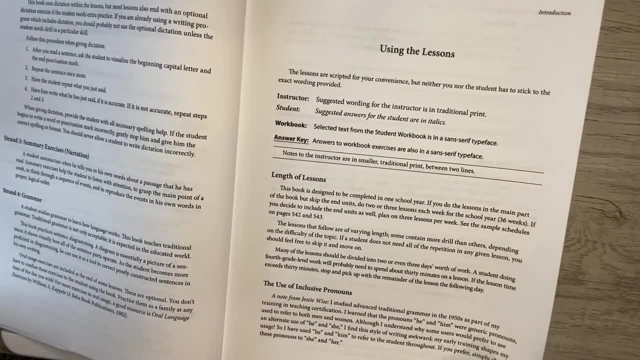 And it says, if you decide to include the units at the end as well, that you'll probably need to do three lessons per week, which is what we do. And it talks about the use of inclusive pronouns, Which is such a funny thing to talk about in this day and age. 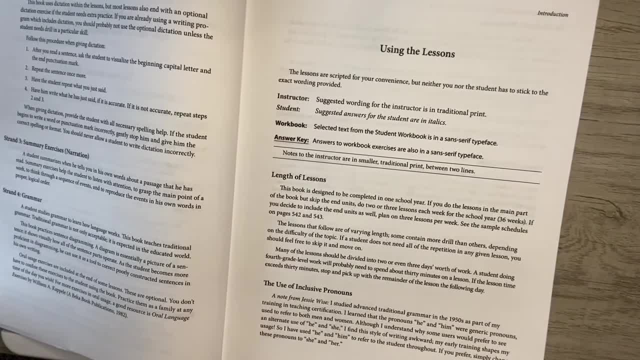 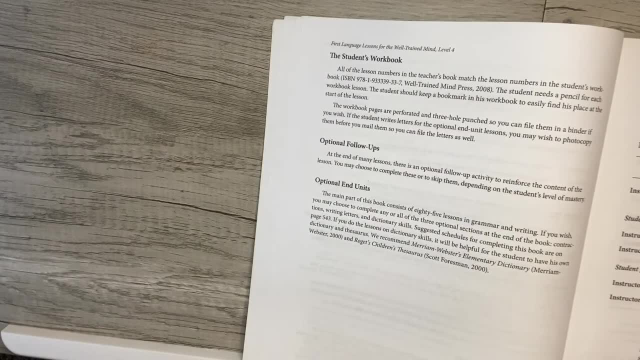 But she does say him a lot. just as you know, traditionally is done Here. this talks a little bit about the student's workbook, the optional follow-ups and the optional end units. Okay, here is lesson one. Again, same setup. 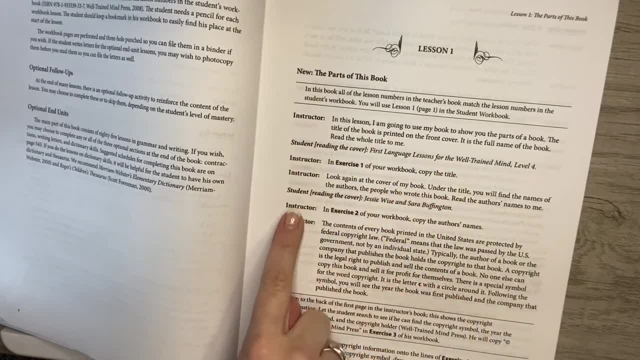 You have instructor, what the student should say, your lines, their lines, Things in boxes kind of like this, are just kind of telling you what to do. And then there's sometimes these optional exercises which, again, I don't usually do. 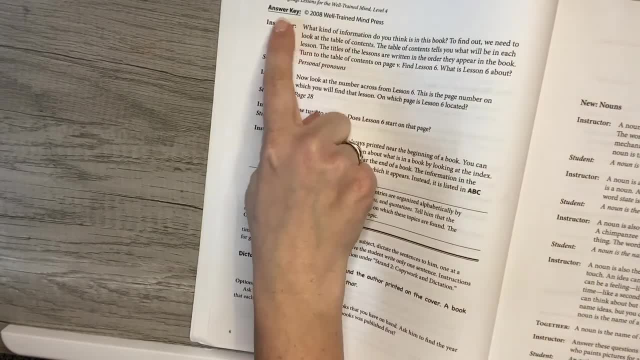 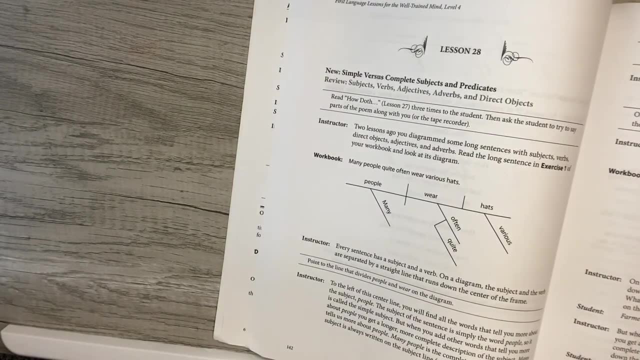 But you very well can. But again, here is an answer key, So the answers are going to be directly into this book, which is really nice. Okay, lesson 28.. Now we are getting into diagramming sentences. So here's simple: versus complete subjects and predicates. 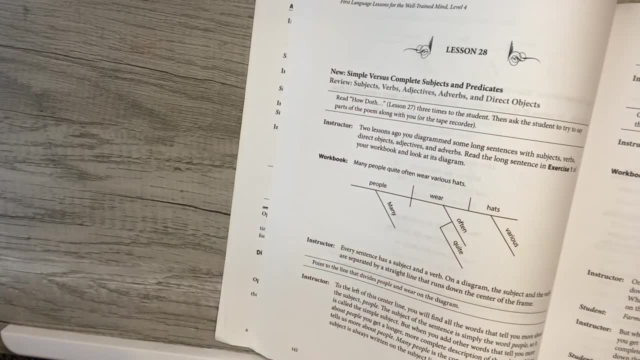 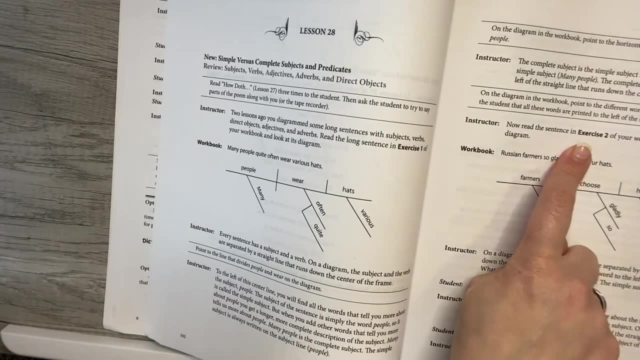 So you'll usually have a little bit of review. It tells you what you'll be reviewing, And then they'll also introduce a new thing. So throughout you will see that they refer to different exercises in bold, And so in your student's workbook that's what theirs are called. 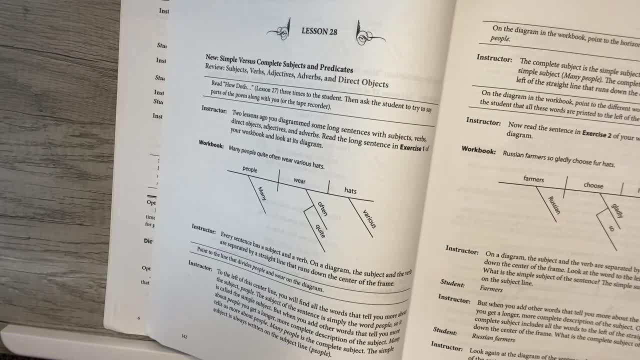 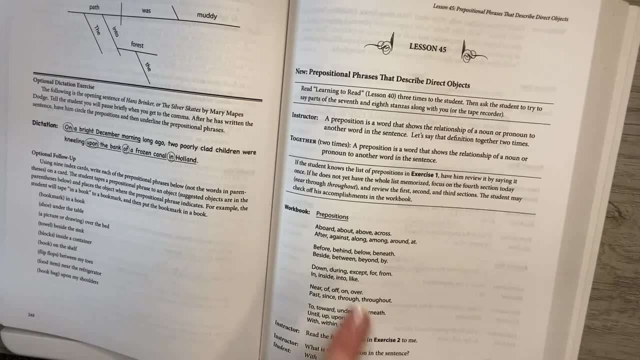 So they'll have exercise one, exercise two. So when you say look at exercise two, they know exactly where to look. Okay, here's lesson 45.. Prepositional phrases that describe direct objects. So you'll work on this list of prepositions. 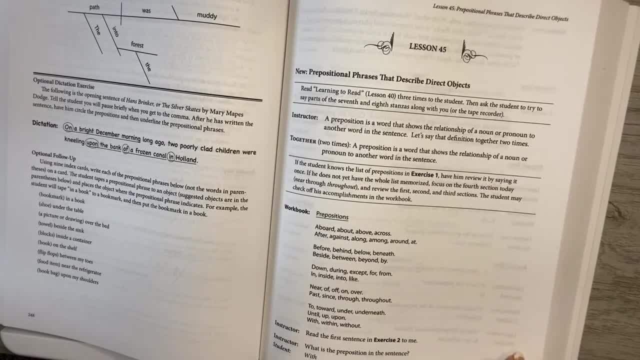 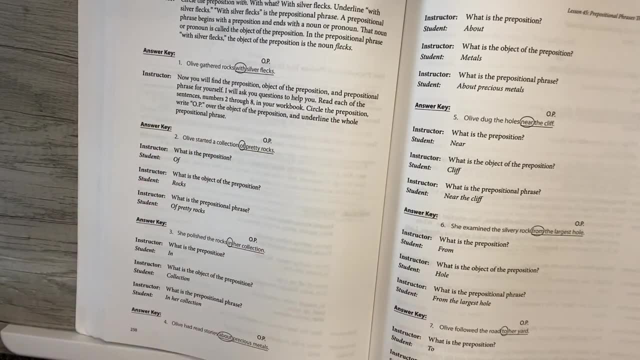 We've been working on this for a long time now. He has them pretty much down by now And again here. this is you telling them what they need to do. They do it, And then there is your answer key, in case you need some help. 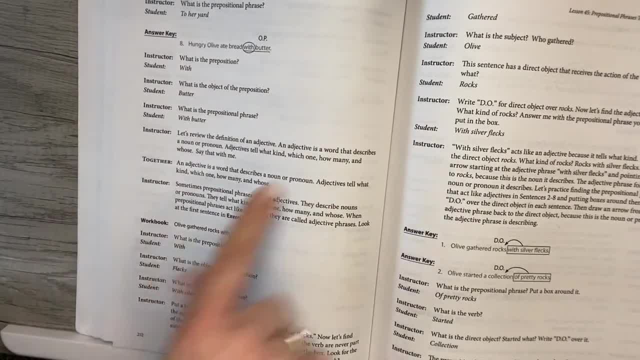 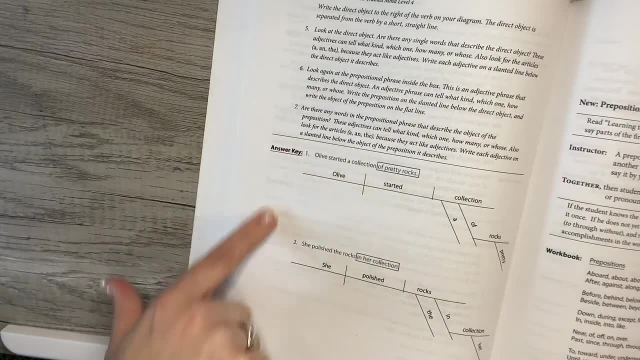 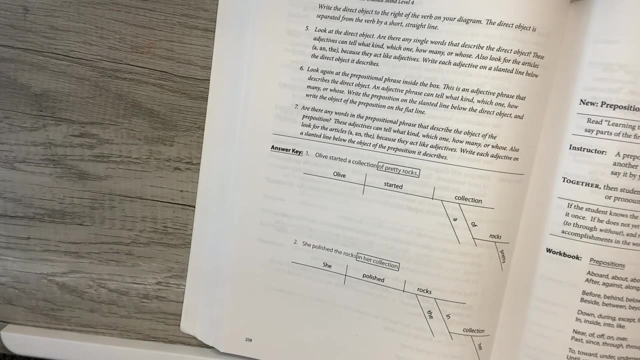 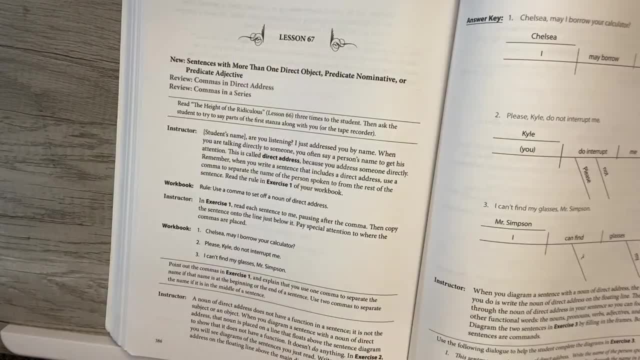 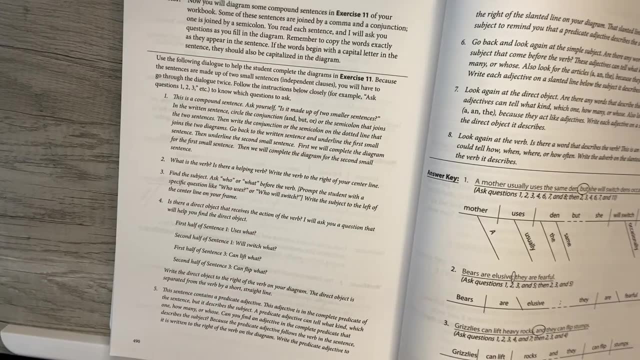 I don't make him do the whole thing. Here's lesson 67.. So again, we're still diagramming, but we're using. you know, we're getting our sentences more complicated as we go. Okay, so this is from lesson 83.. 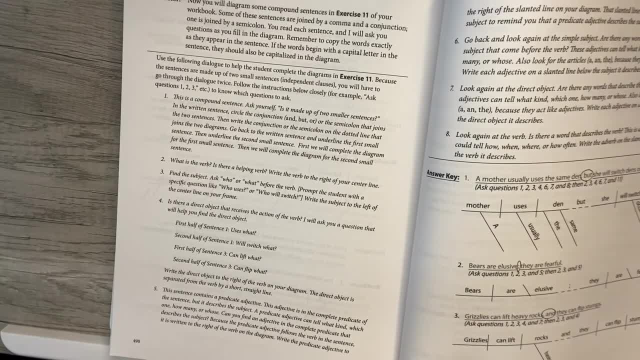 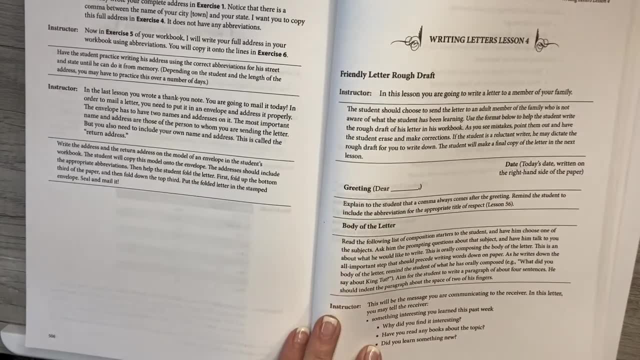 Where we are reviewing, And so these are some really complicated sentences that you will have them diagram And then here toward the back, I was going to show you kind of what those writing letters lessons looked like. So it just tells them what you need to do to write a good letter. 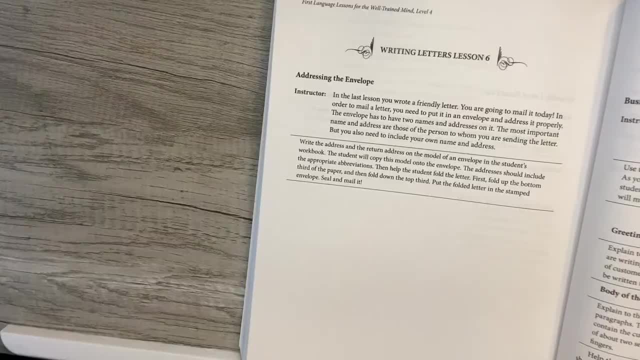 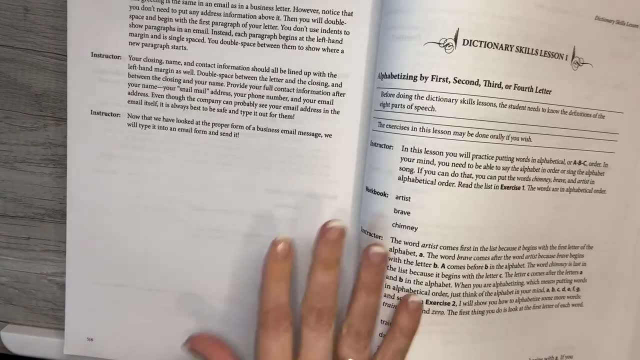 And then, of course, they actually write letters and send them to family members. It talks about even addressing the envelope and what that needs to look like, And even talks about business letters. And then we're talking about our dictionary skills. So we're talking about alphabetizing. 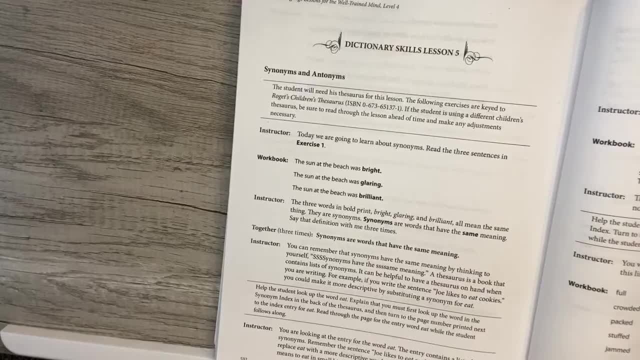 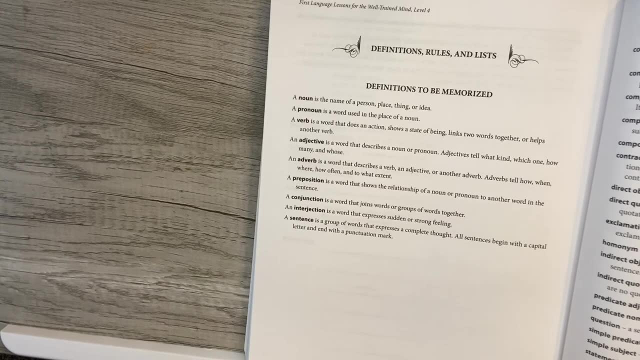 what parts of speech the words are in that we look up, And then here we're talking about synonyms and antonyms in the dictionary. Okay, then here at the end you have definitions, rules and lists, So definitions that they're supposed to memorize. 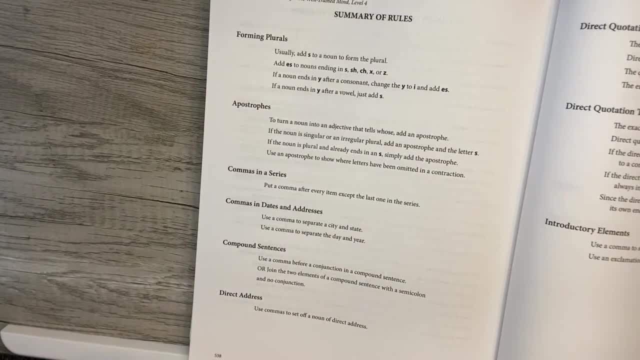 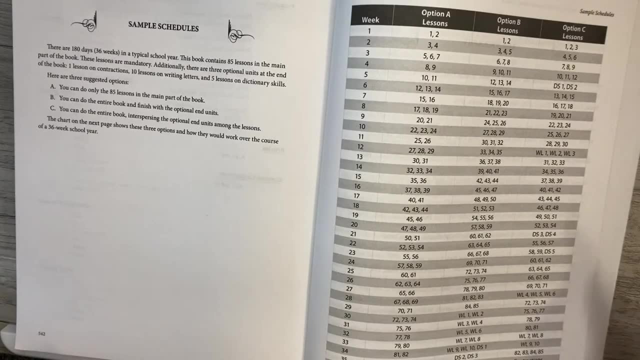 A glossary of terms to know, A summary of the rules Lists that they should memorize. And then here you have a sample schedule. Here is the schedule we use Down here along this side. option C, So option A- is when you just want to do. 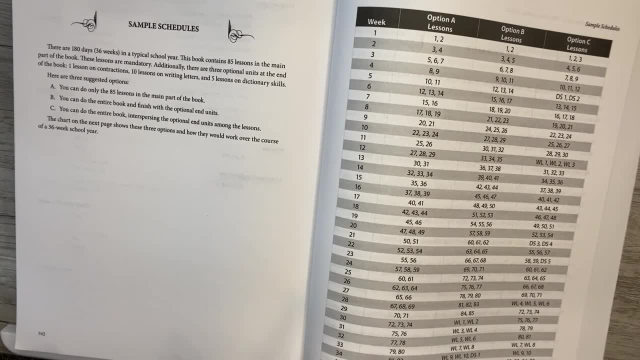 the main 85 lessons of the book. So you're usually doing- you're alternating- two and three lessons a week. Option B is where you do the entire book and then finish with those optional end units, And then option C, which is what I do. 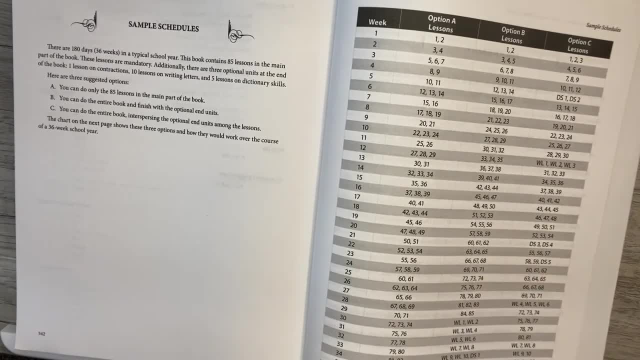 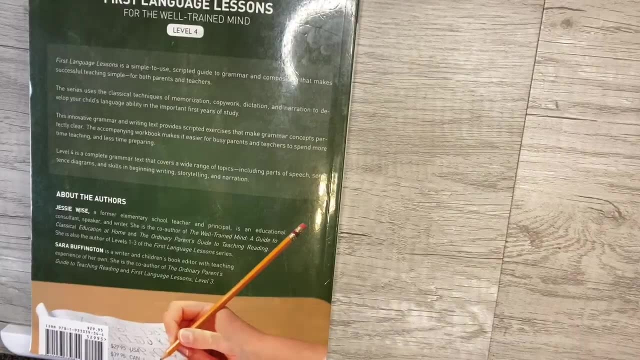 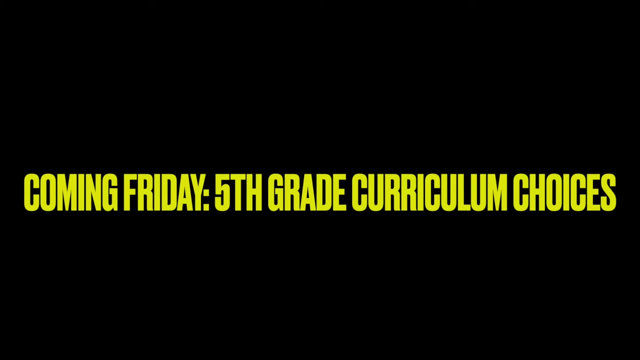 is where they mix in those units kind of throughout the year. And then here's your bibliography, So all your sources and your index. So comment down below with what curriculum you use for grammar. Be on the lookout. Friday I have a fifth grade curriculum choices. 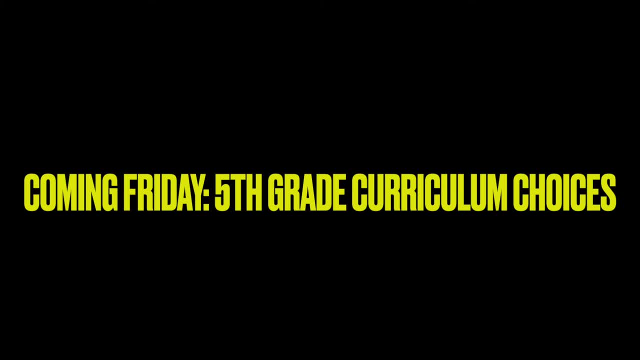 for the 2021-2022 school year And subscribe if you haven't already, And I thank you so much for watching. Bye. 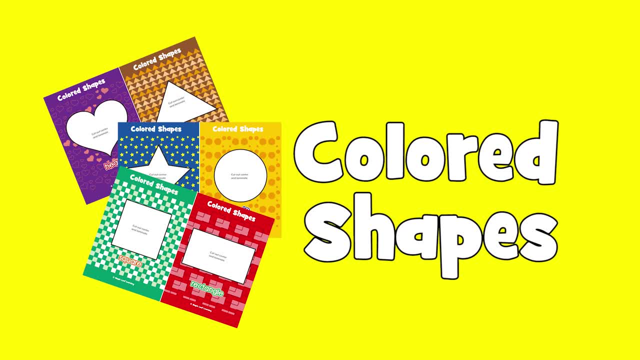 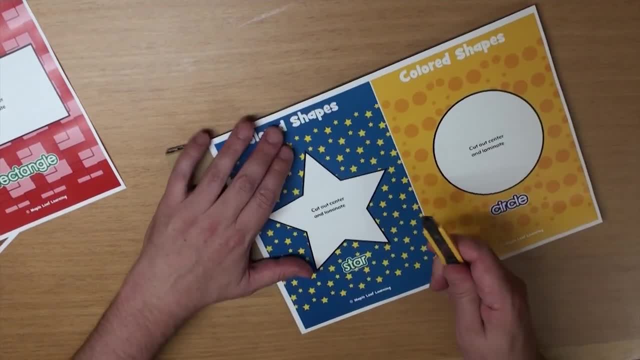 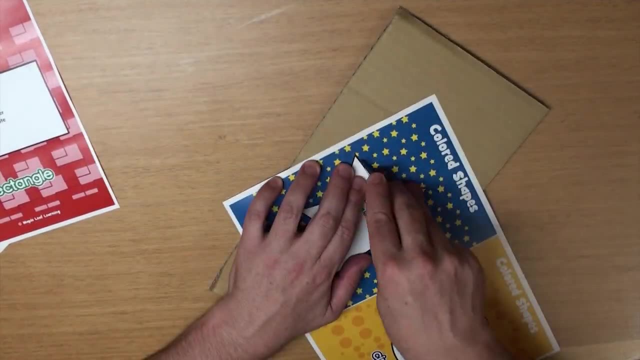 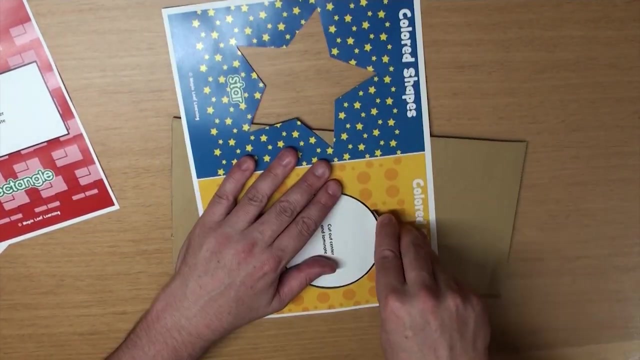 The colored shapes activity. Well, print out all of your shapes like this and grab yourself a cutter knife and we're going to cut out the insides of all of these shapes. okay, Be careful. There's the star and the circle, and please do the same with all of the other shapes. okay, 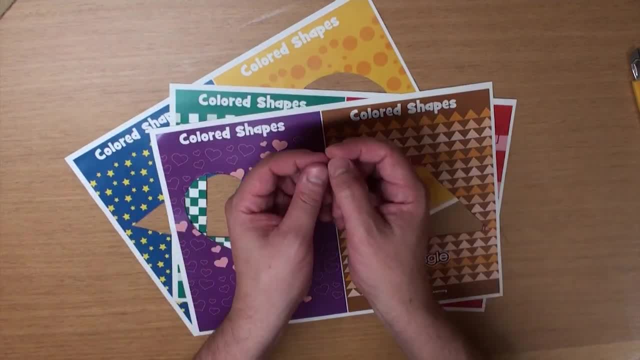 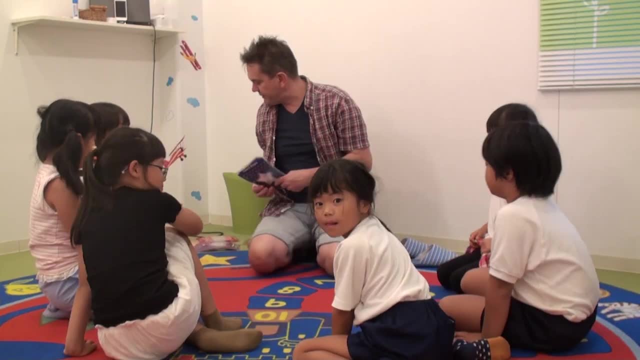 Now cut them out and cut off the edges, and you're going to need to laminate them. okay, Now we're ready to play. Okay, guys? Anyways, today I brought some shapes, and the first one you have to do- what shape is this? You know it's a star, Good job. So here's a star for you.